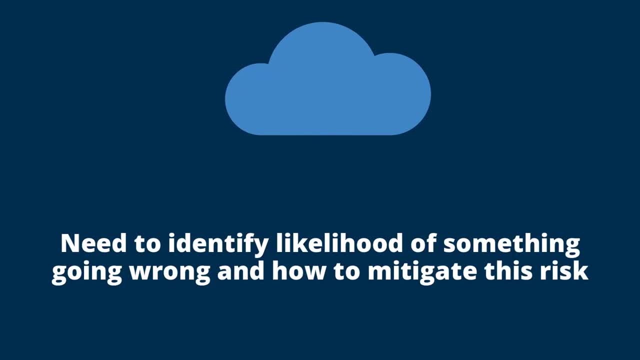 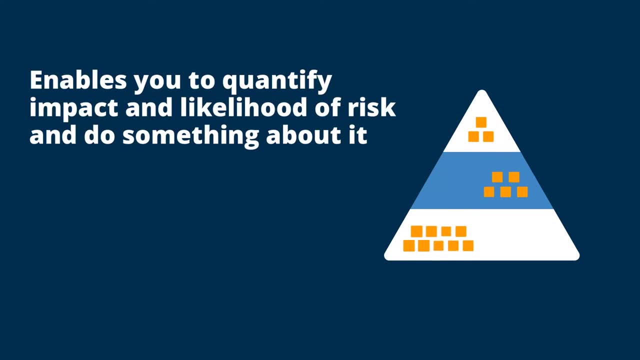 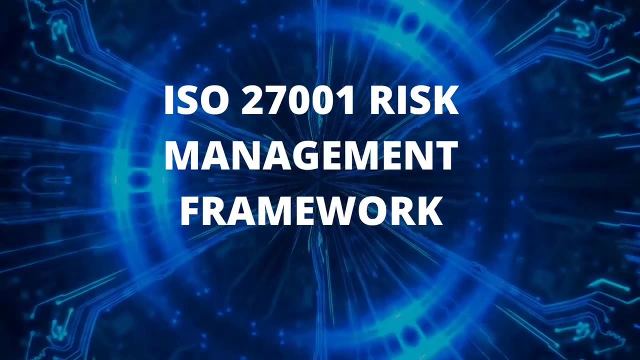 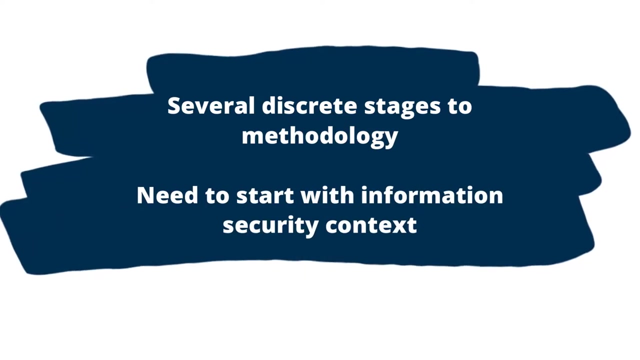 likelihood of something going wrong and what can be done to mitigate this risk. In a nutshell, it enables you to quantify the impact and the likelihood elements of information security risk and then go on to do something about it. ISO 27001 risk management framework. There are several discrete stages of an ISO 27001. 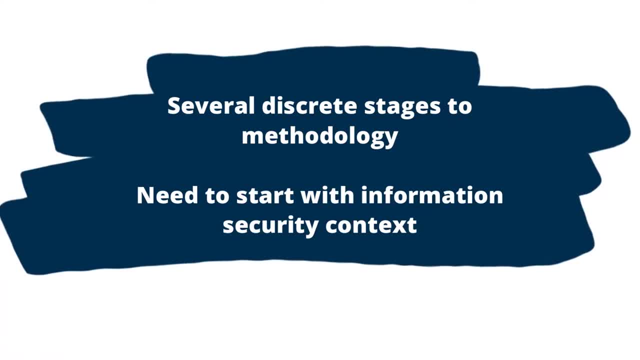 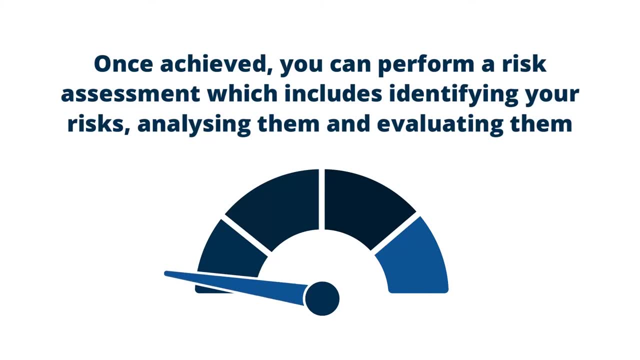 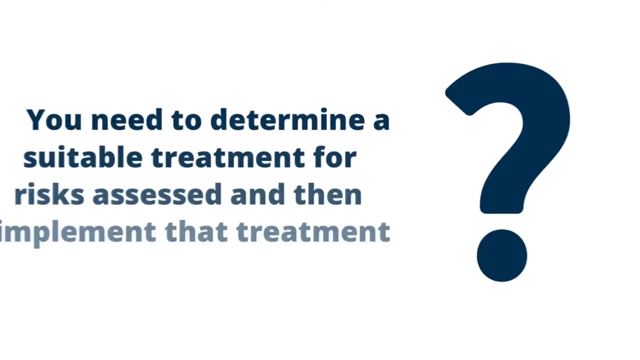 risk management methodology. First of all, it is important to understand the information security context of your organisation. Once this has been achieved, you can perform a risk assessment, which includes the need to identify your risks, analyse them and evaluate them. You then need to determine a suitable treatment for the risks you have assessed and then implement. 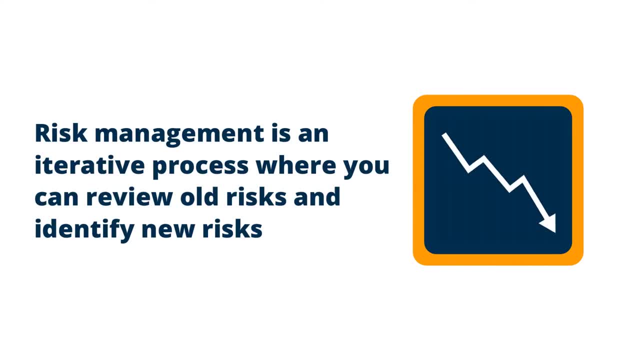 that treatment. It is vitally important that you do not see this as a one-off exercise. Your risk management methodology should be designed to be iterative. This enables you to not only review the status of risks you have previously identified, taking into consideration any potential changes in context, but it also enables you to identify new risks. 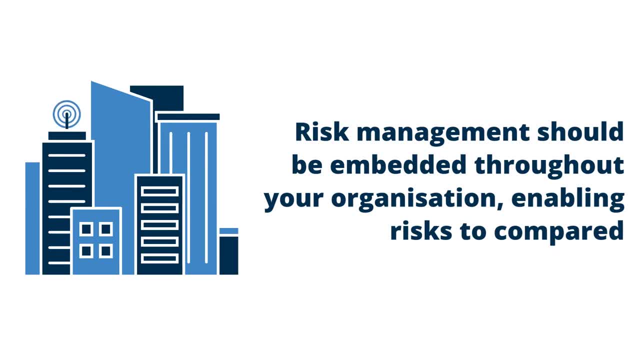 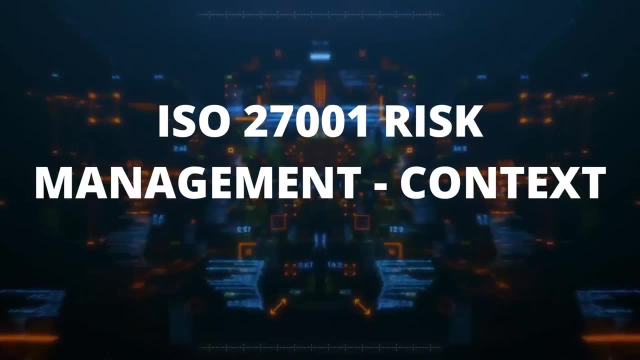 The high-level stages of a risk management methodology, as described above, should be thought of as a framework that enables risk management to be embedded within key processes throughout your organisation so that any identified risks are comparable. ISO 27001 risk management context- The first stage of your risk management methodology. 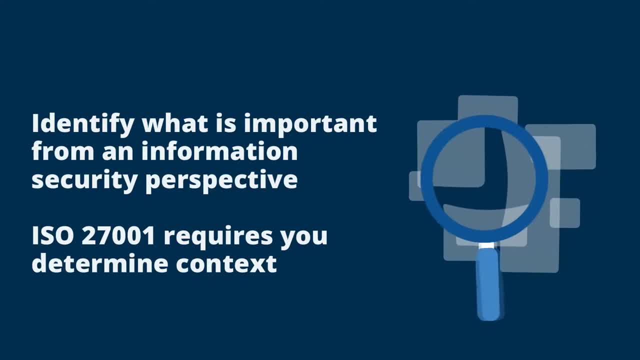 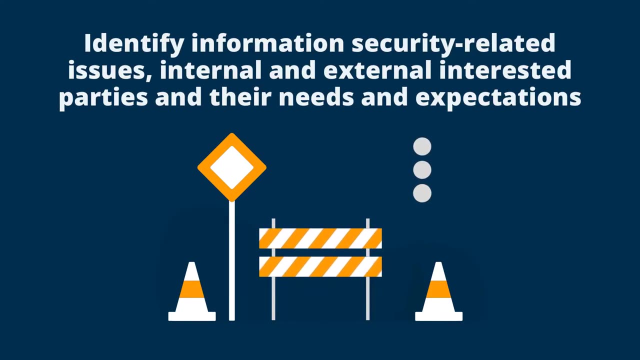 needs to identify what is important to you or your organisation from an information security point of view. ISO 27001 requires you to determine the context of your organisation, part of which means that you need to be able to identify the information security related issues that you face, along with who the internal and external interested parties are and what. 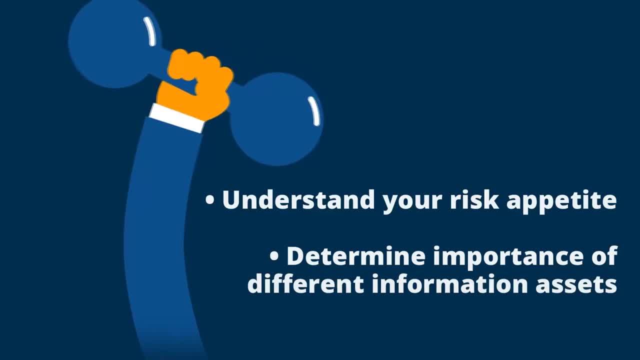 their needs and expectations are. It is important to also understand what your risk appetite is at this stage and what your risk appetite is at the end of the day. You need to be able to identify what your risk appetite is at this stage and what your risk appetite is at the end of the day. 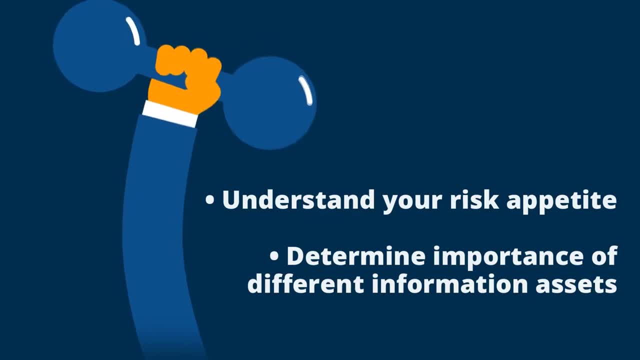 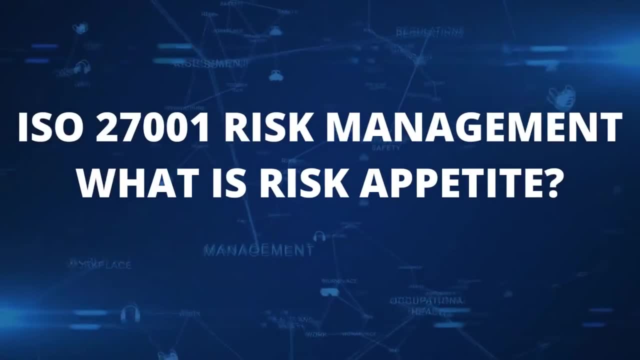 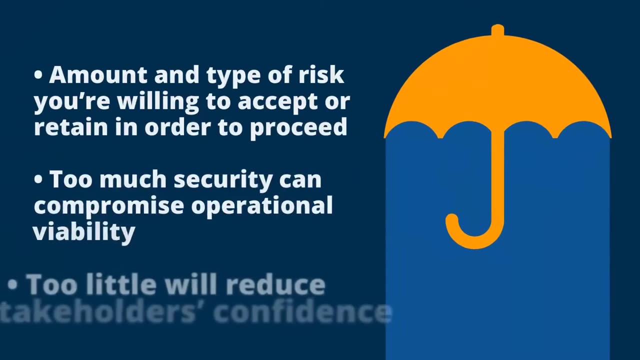 Thisivack & Jakes. ISO 27001 risk management. What is risk appetite? Risk appetite is simply the amount and type of risk you are willing to accept or retain in order to allow businesses operation to proceed. This is important because too much security can sometimes compromise your future. equal short term impact. 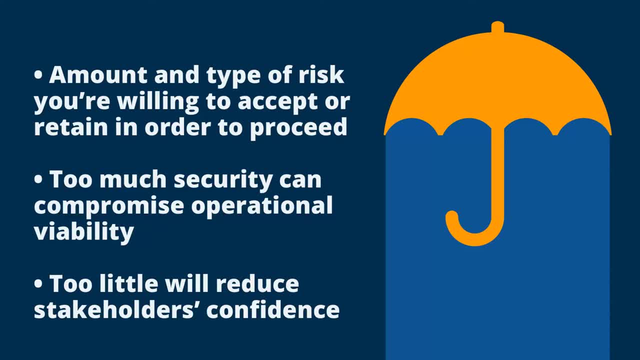 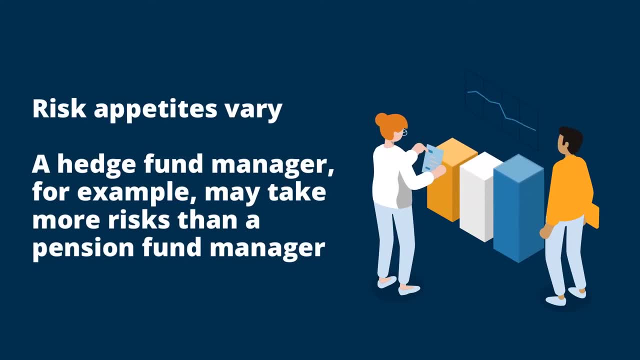 your operational viability, whereas too little will reduce the confidence of your stakeholders. Some types of organisations are willing to accept more risk than others. For example, a hedge fund manager is likely to take more risk in order to make greater profits over a short space of time, whereas a pension fund manager generally prefers a less risky, steady growth. 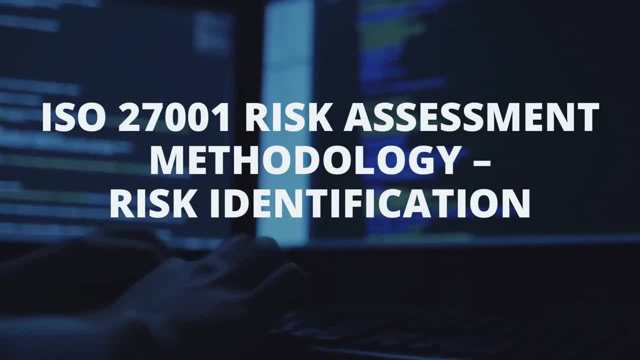 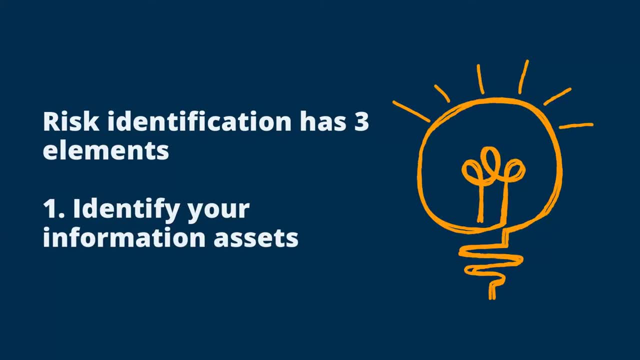 approach: ISO 27001 risk assessment methodology- Risk identification. Once you have determined the context, you can go ahead and conduct a risk assessment. The first part of a risk assessment is to identify the risks that you face. This can be broken down into three elements. The first: 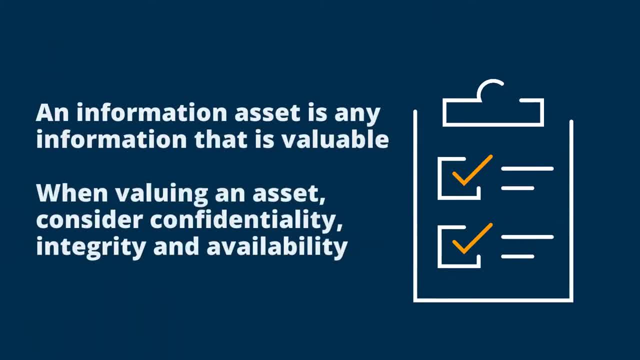 element is to identify your information assets. An information asset is any information that has value to you. There are several different ways to calculate the value of your information. It is important that you not only consider the confidentiality needs of the information, but also the integrity and availability requirements. The second element of risk. 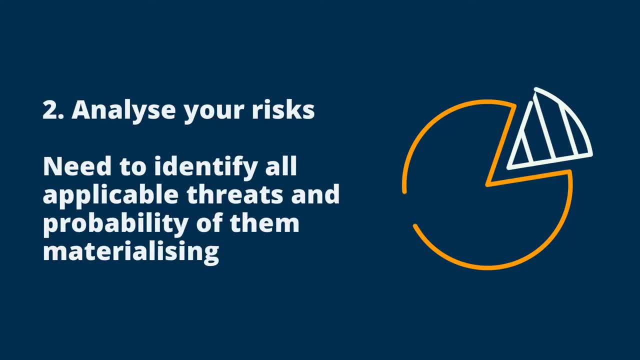 identification is threat analysis. You need to have a process which enables you to identify all of the threats which are applicable to the assets you have identified. If a particular threat is applicable, then it is also a good idea to think about how probable it is that the threat 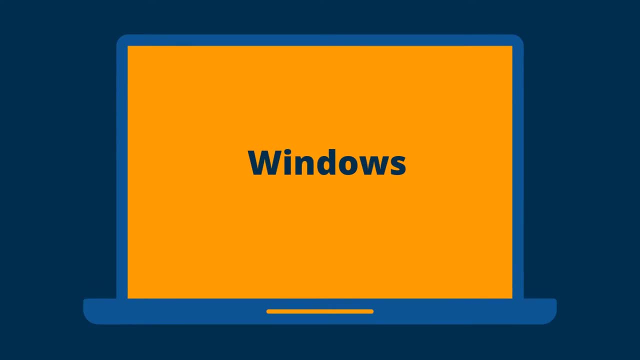 will materialise. If a threat is applicable, then it is also a good idea to think about. For example, if you use Windows-based computer systems which are connected somehow to the internet. the probability of them being affected by a virus is probably very high if you do. 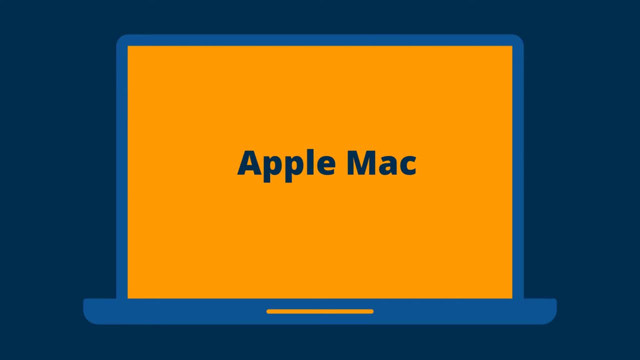 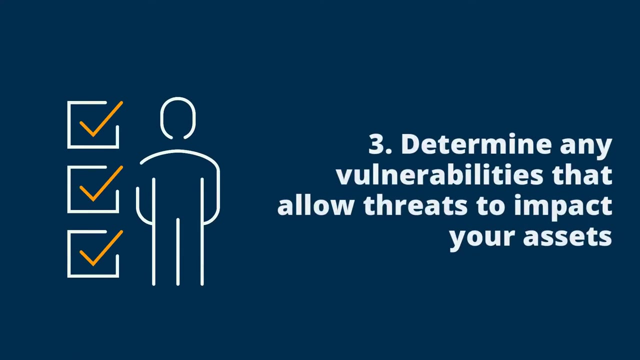 nothing to stop it, whereas if you are using an Apple Mac, which is never connected to the internet, the probability is very low. The third element of risk identification is the need to determine if there are any vulnerabilities that would allow a threat that you have identified to cause an impact on your asset. 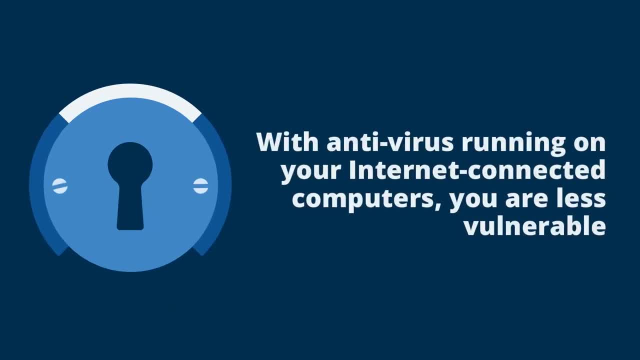 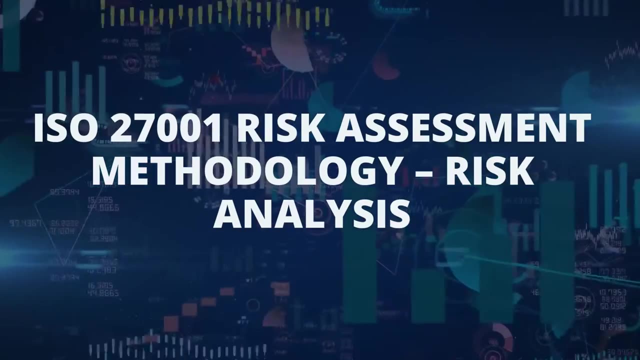 To carry on with the example we have just used, if you have an antivirus system installed and running on your internet-connected Windows computers, you are less vulnerable to this particular threat than if you didn't. ISO 27001 Risk Assessment Methodology- Risk Analysis. 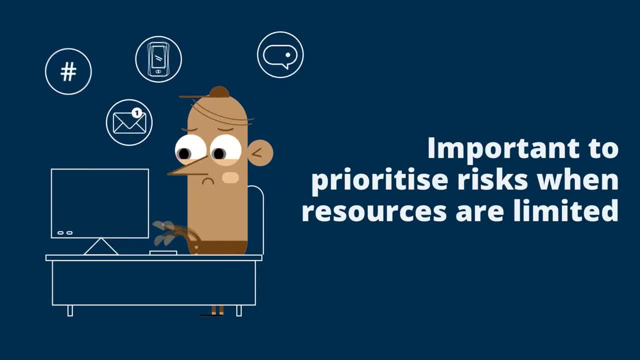 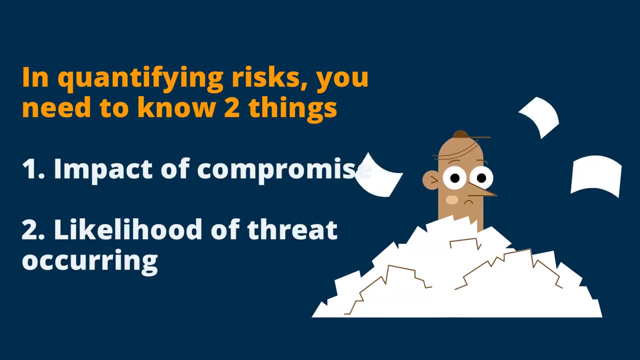 One of the useful aspects of the output from an effective risk assessment is the ability to prioritise your risks. This is important, as you may not have sufficient resources to fully mitigate every risk that you identify. This means that it is important to somehow quantify your risks. 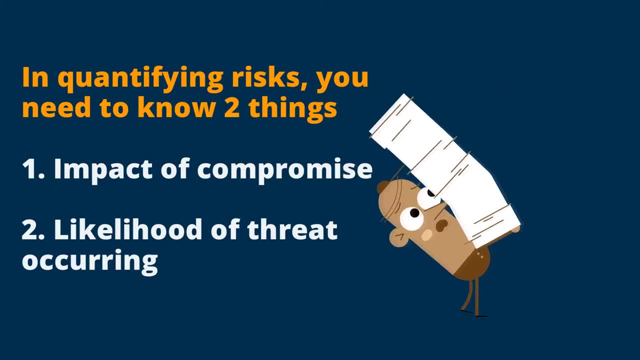 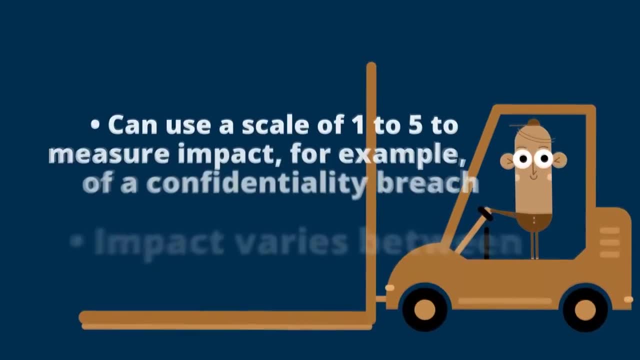 To do this, we need to know two things: First, how much of an impact would be felt if a compromise occurred and second, what is the likelihood of that threat occurring. One good idea is to use a set of scales to record values in these areas. 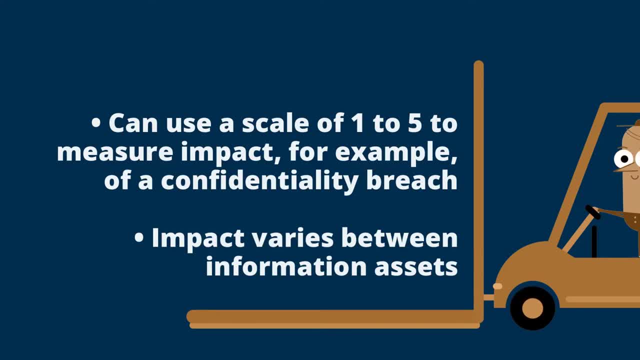 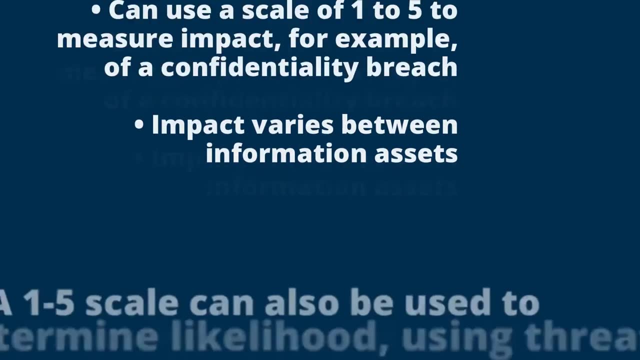 For example, using a scale of 1 to 5, we could say how impactful it would be if the confidential of an asset were breached. Clearly, breaches of confidentiality would cause a greater impact for some assets, for example HR records, than others like the staff canteen menu. 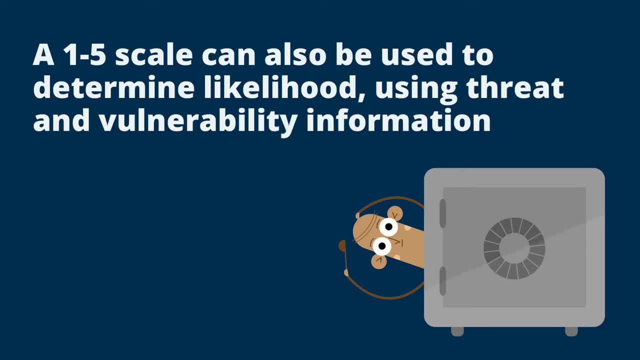 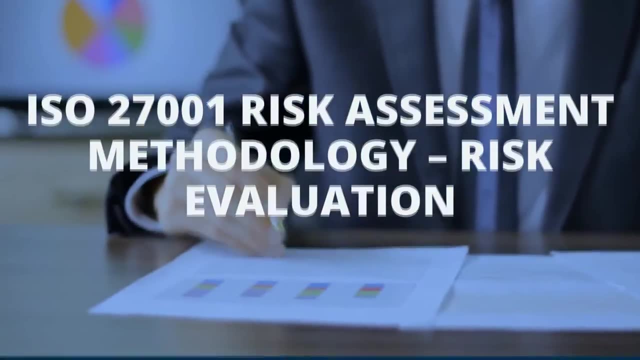 A second 1 to 5 scale could be used to determine the likelihood of a breach occurring, and we would take into consideration the threat and vulnerability information we spoke about earlier. in order to do this. ISO 27001 Risk Assessment Methodology- Risk Evaluation. 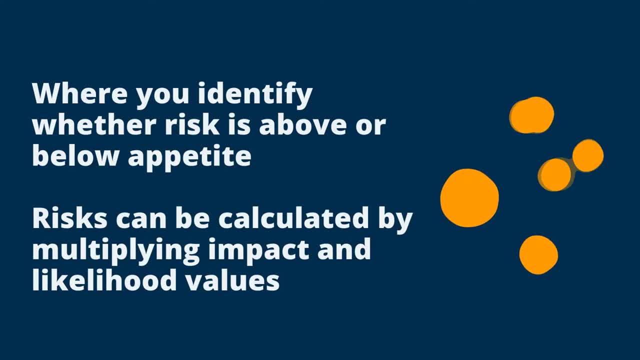 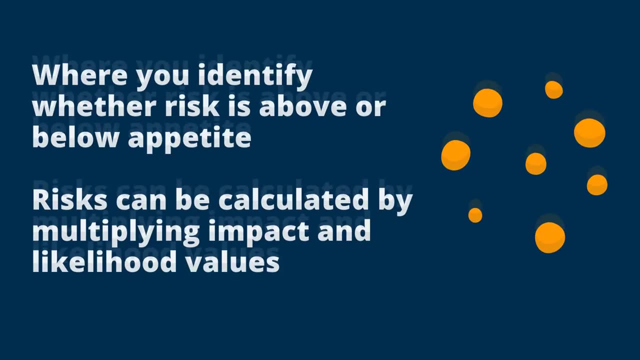 Risk evaluation is a relatively simple process, as it requires you to identify whether or not the risk that you have identified is above or below appetite. To do this, the first thing we need to do is calculate the value of the risk, which simply means multiplying the impact and likelihood values together. 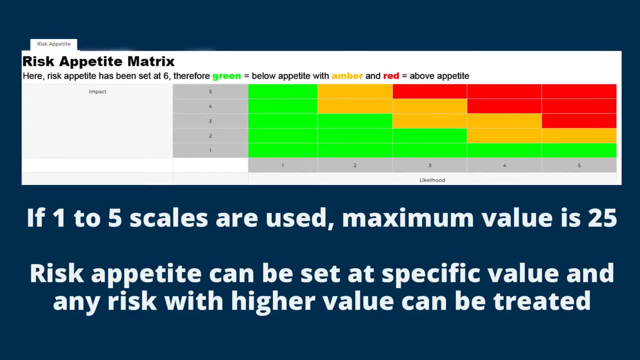 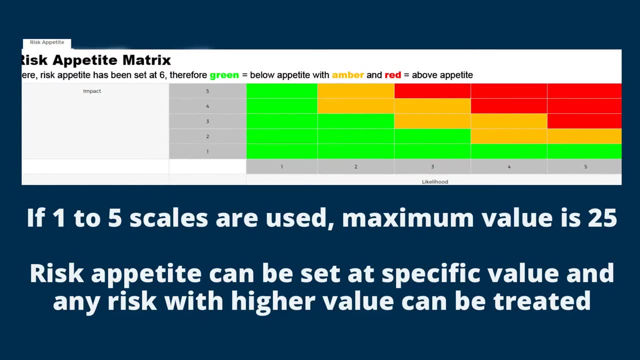 We have a range of possible values, which result from multiplying the two 1 to 5 scales together. The appetite is stated within the methodology. If a particular risk is above this value, then it is above appetite, which means that it can then be flagged for treatment. 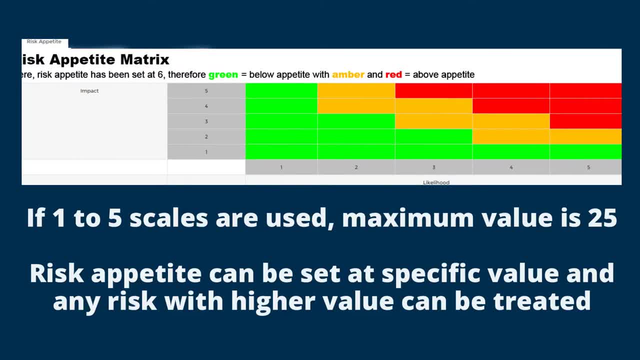 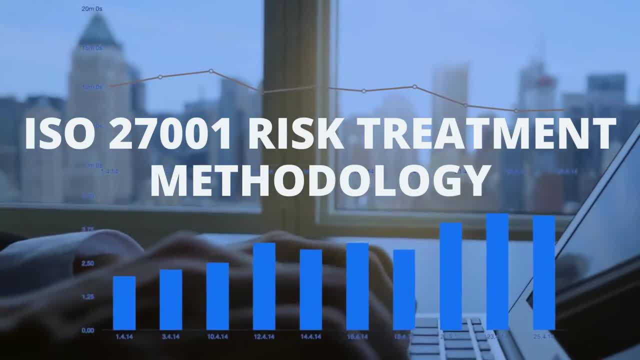 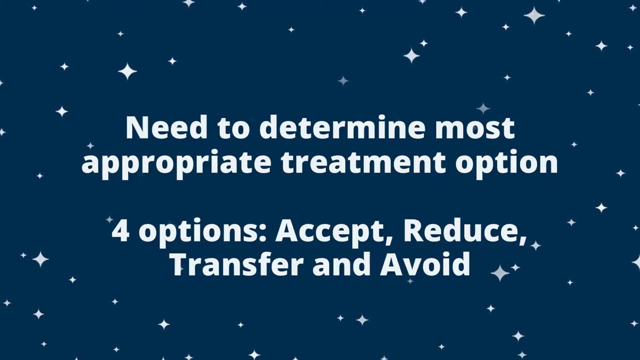 Anything below appetite can be accepted and monitored for change. ISO 27001 Risk Treatment Methodology. Your risk management methodology needs to include a methodology for determining the most appropriate treatment for the risks that you have identified. The risk management methodology needs to include a methodology for determining the most appropriate treatment for the risks that you have identified. 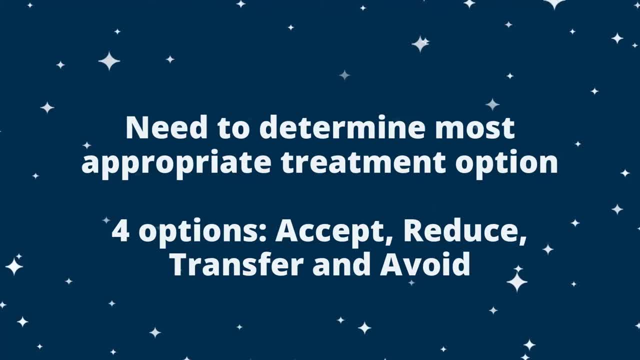 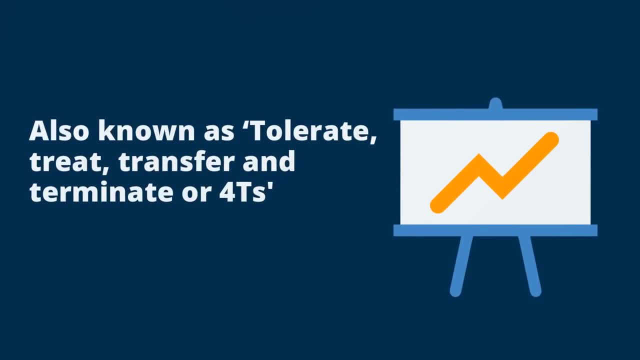 There are four possible treatments to choose from. These are Accept, Reduce, Transfer and Avoid. You may come across different terms used for these, such as Tolerate, Treat, Transfer and Terminate. This example is known as the four T's. however, they take the same approach. 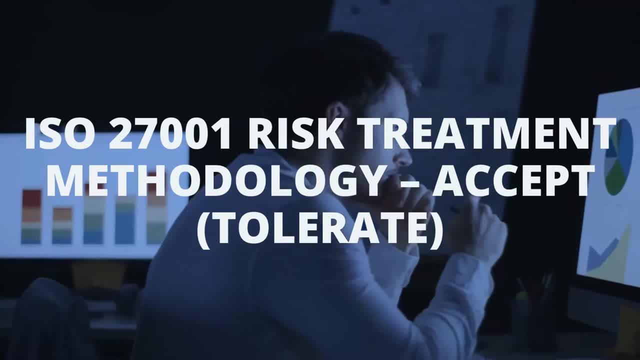 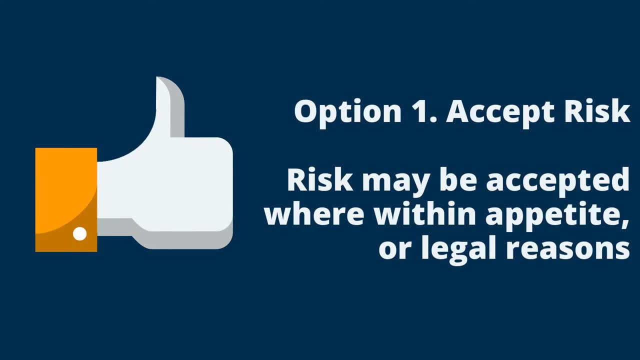 ISO 27001 Risk Treatment Methodology- Accept or Tolerate. One of the four treatments provides you with the ability to accept or avoid risk. The risk management methodology is the risk management methodology. We have already seen that this is possible, as it is likely that you will simply accept. 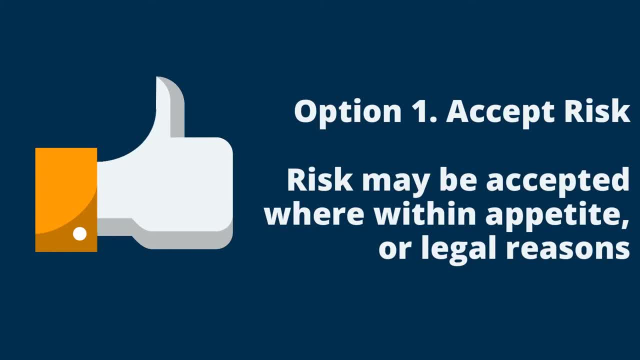 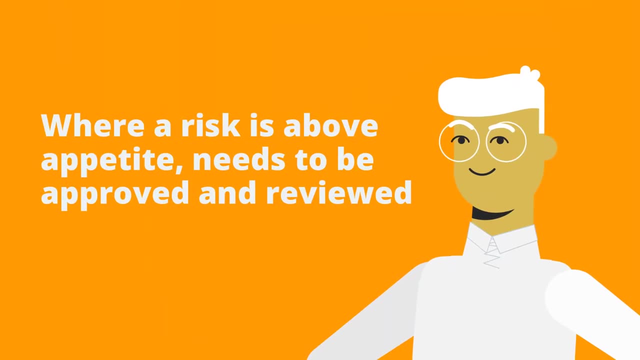 risks that are below appetite. However, you can also make an informed decision to accept risks in certain circumstances, such as where there is a legal requirement preventing you from taking the desired action or you have insufficient resources to do so. These cases should be few and far between, though, and should always be approved by appropriate 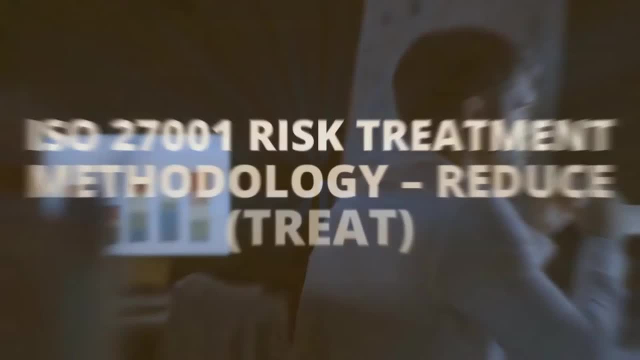 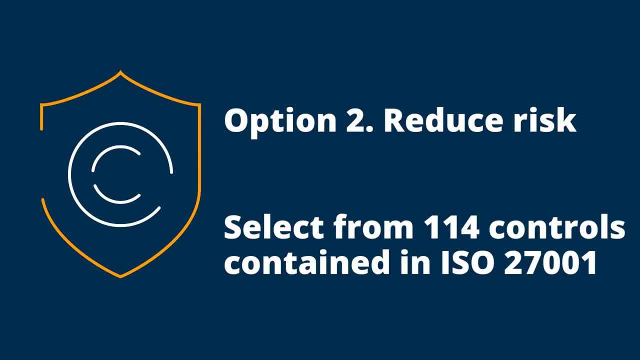 Reduce or Treat. The second treatment option is to Reduce or Treat the risk. This is done through the implementation of controls. ISO 27001 provides you with a list of 114 best practice controls that can be used to mitigate the risks that you have identified. 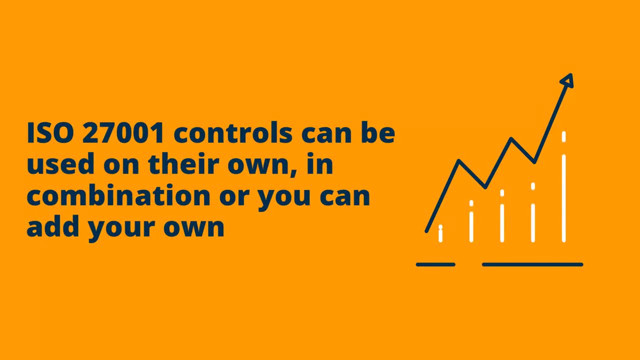 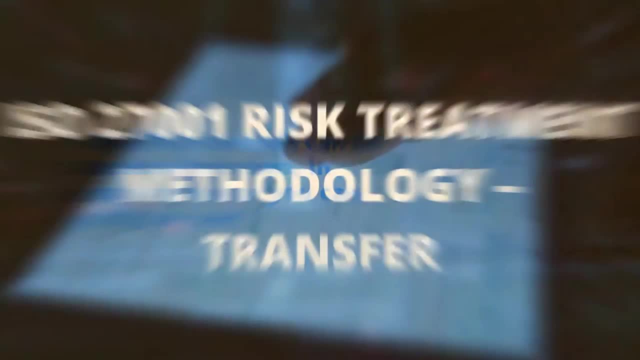 These can be used in combination in order to increase their effectiveness and, of course, you can also add controls of your own that do not appear in the list. So let's take a look at the list. 1. Reduce or Treat the risk in ISO 27001. ISO 27001: risk treatment methodology- transfer the third risk. 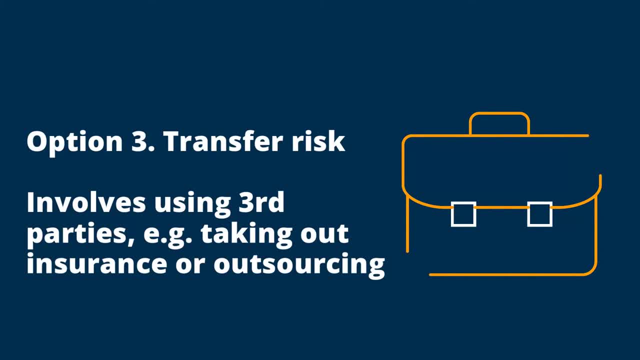 treatment option is to transfer the risk. the transfer option involves the use of third parties to help you mitigate your risks. you could do this, for example, by offloading some of the financial impact of something going wrong by taking out an insurance policy. another way of doing this is to outsource the responsibility. 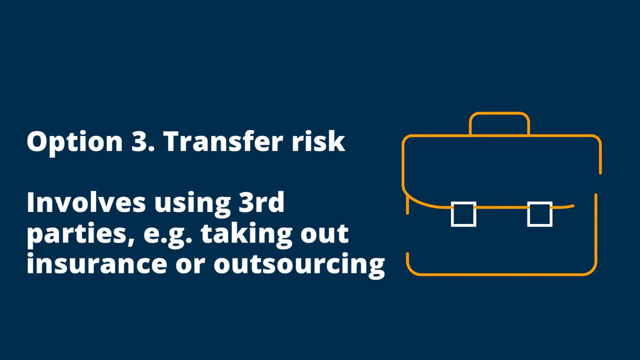 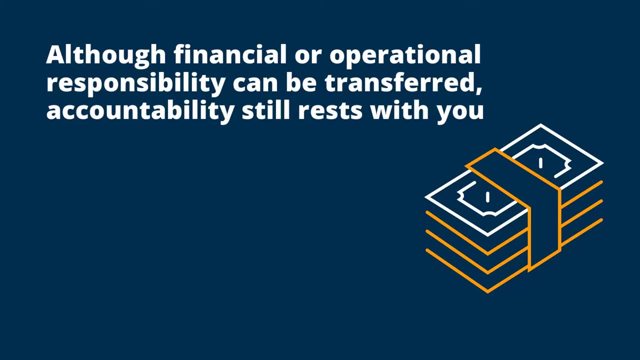 for implementing and operating technical controls to a third party, such as an IT managed service provider. it is important to note here that although responsibility for financial impact or the management of operational controls can be transferred to a third party, the accountability associated with the risk cannot. in other words, you will still be held accountable by your stakeholders if 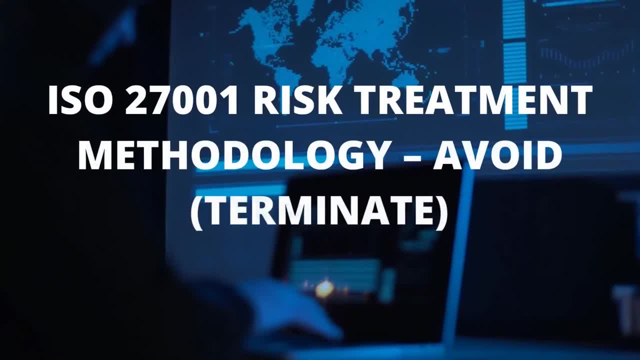 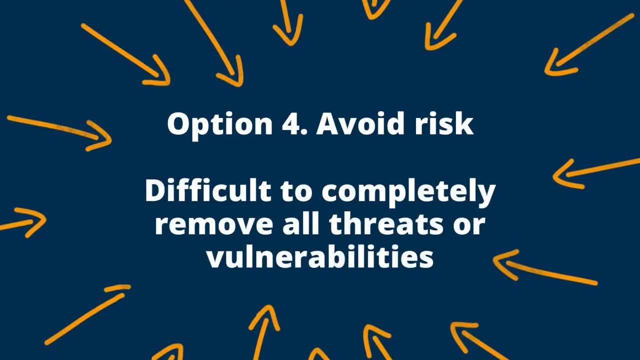 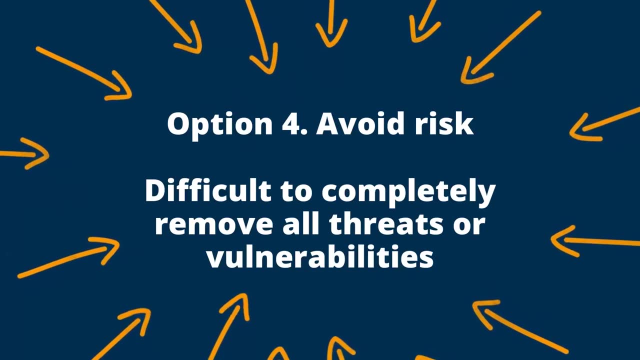 something goes wrong. ISO 27001 risk treatment methodology transfer. the risk relationship with the risk is to ensure, avoid or terminate. the fourth risk treatment option is to simply avoid the risk. as we have discussed before, there are three component parts to risk: the impact felt by the organization. 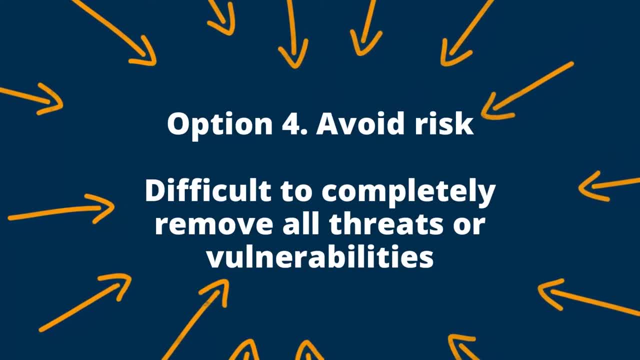 following a breach of confidentiality, integrity or availability for an information asset, a threat that could cause this impact and a vulnerability that would allow it to do so. it is possible to avoid risk completely by eliminating one or more of these three elements. however, it is unlikely that we would be able to completely remove all threats or all vulnerabilities, which leaves us. 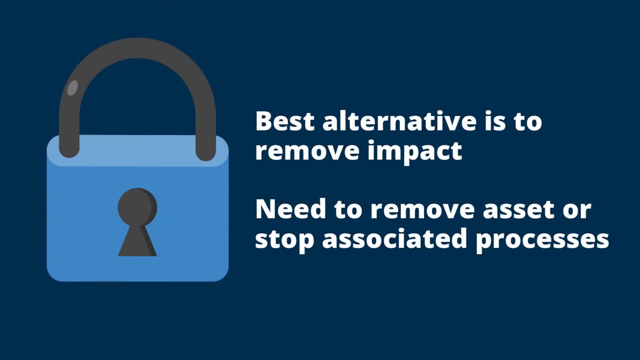 only with one viable option, which is to remove the impact. this is done by removing the asset or stopping the processes that are associated with the identified risk, for example, to avoid the risks associated with the taking of credit card payments, removing that process and only deal in cash. there are obvious issues associated with taking this. 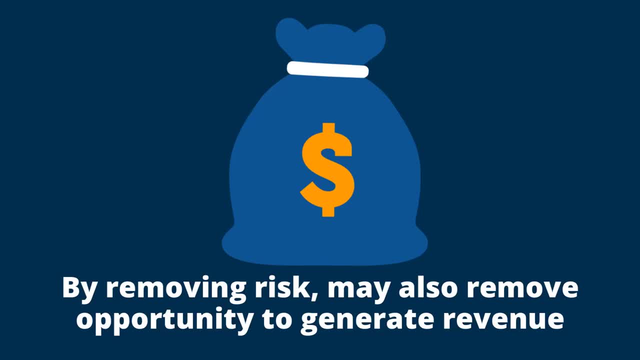 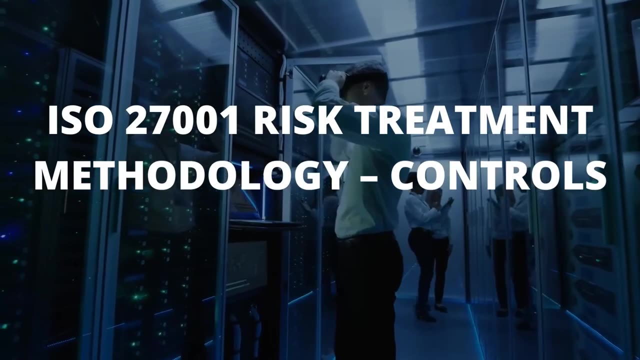 approach, as it is unlikely to be looked upon too favorably by your stakeholders, especially if the process is revenue generating. this is the reason why this particular risk treatment methodology is really used. ISO 27001 risk treatment methodology controls the most common option chosen to treat risks other than may be accessible. 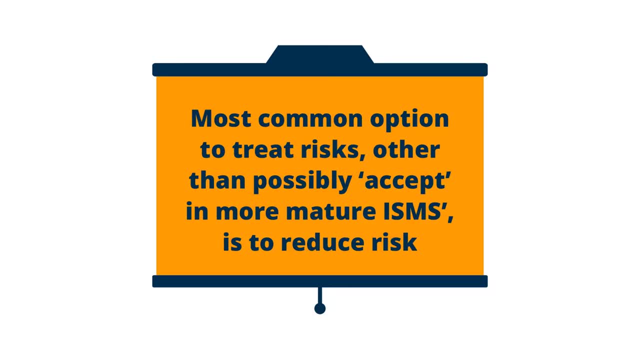 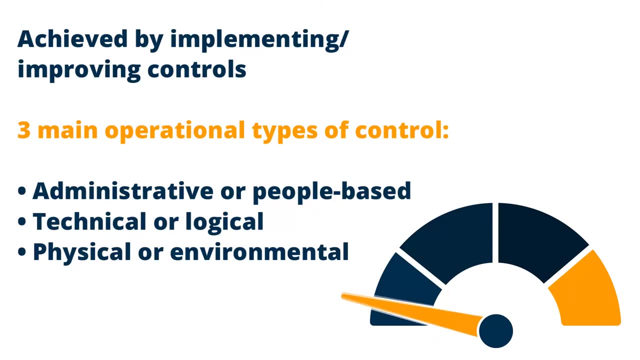 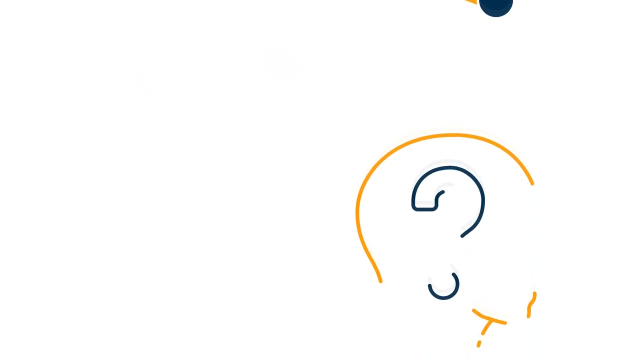 in more mature is mss is to reduce the risk. this is done by implementing controls or improving existing ones to address the risk. there are three main operational types of control: administrative or people-based controls, technical or logical controls and physical or environmental controls. within these three operational types, there are several different tactical uses of controls, such 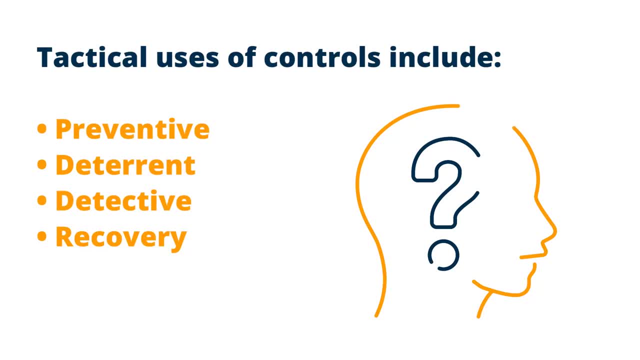 as those that are designed to prevent a threat from materializing, those that are designed to deter people from carrying out an undesired action, those that detect if a threat has materialized or those that enable you to recover from a situation after the threat has been dealt with. and there are several others operational types and tactical. 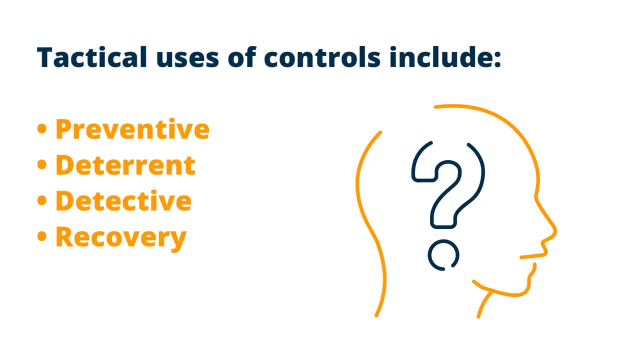 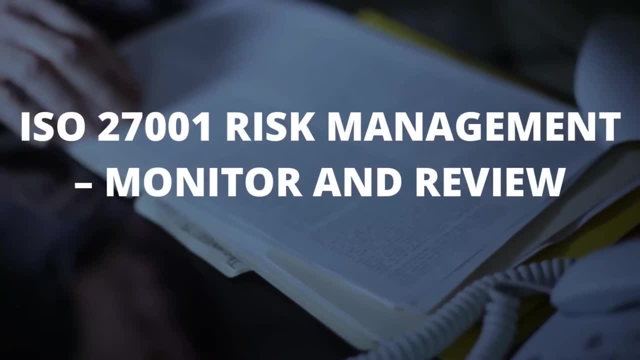 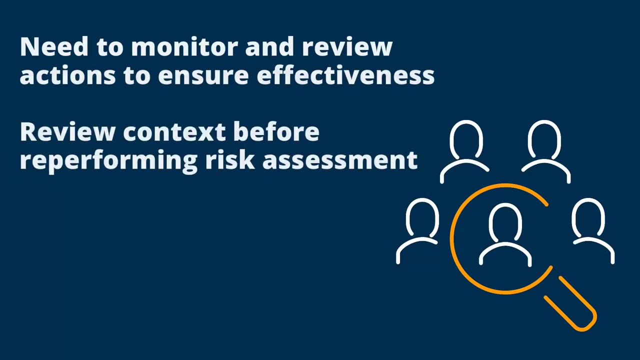 uses of controls are not mutually exclusive and can and should be used, where possible, in combination to provide a greater depth of security. ISO 27001- risk treatment methodology. ISO 27001- risk management, monitor and review. it is important to ensure that any actions you take to address the risks you have identified are monitored and reviewed to ensure that they have. 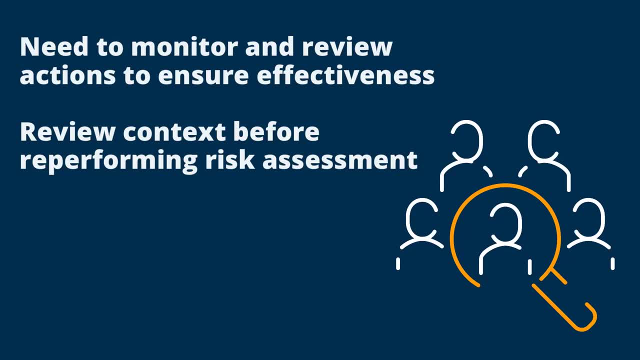 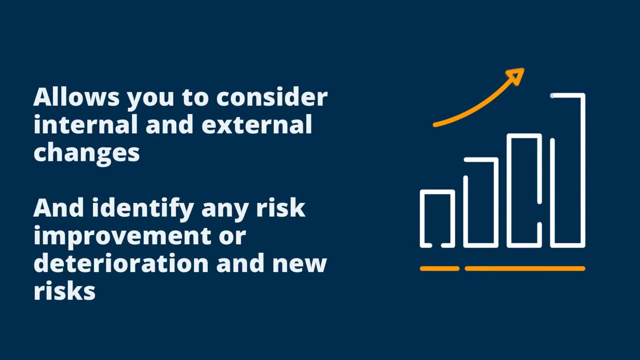 the desired effect. part of the monitor and review process should also include a review of context before the risk assessment is re-performed. this will allow you to identify and take into consideration any changes that may have happened either internally within your organization or externally, such as changes. 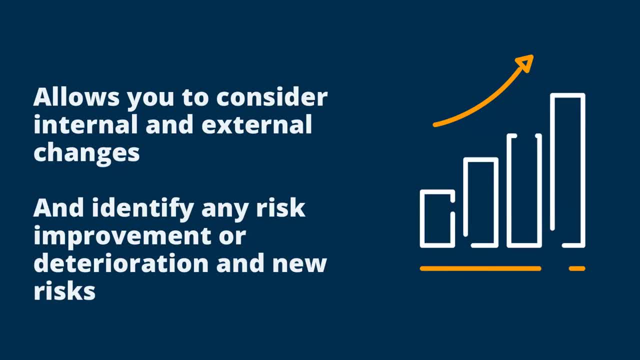 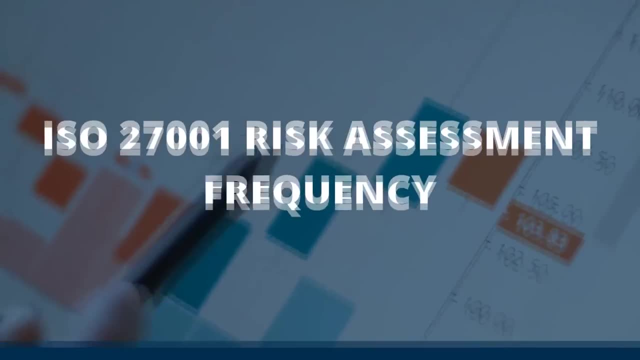 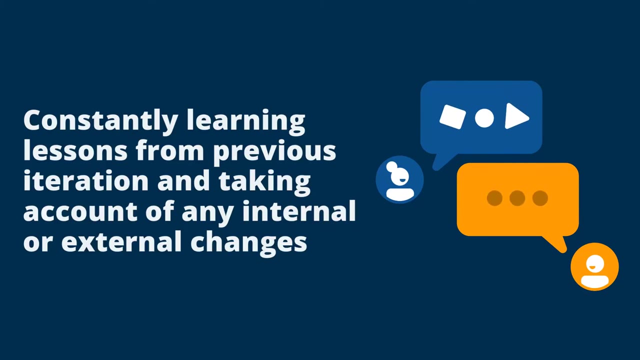 in legislation or changes to the threat environment. thus, you are able to identify if risks that have previously been identified are getting worse or, hopefully, better, and you will also be able to identify any new risks. ISO 27001 risk assessment frequency. risk management and therefore risk assessment, is an iterative process and each iteration should take into consideration lessons. 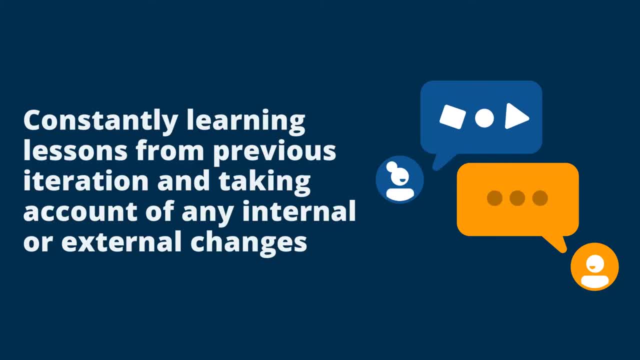 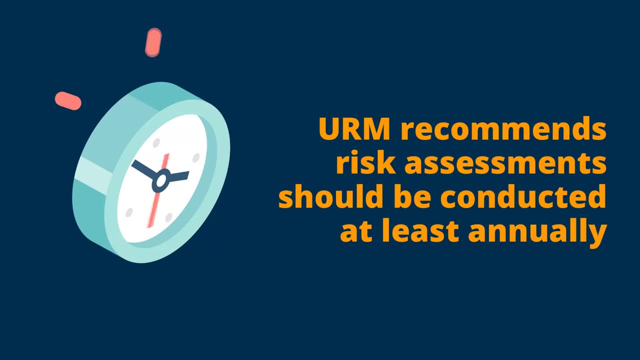 learned from the previous iteration and should take into consideration any internal or external changes, thus enabling continual improvement. there is no hard and fast rule on the frequency of risk assessment, but URM recommends that the frequency is no less than annual. this does not necessarily mean that you should set aside a certain amount of time at a certain 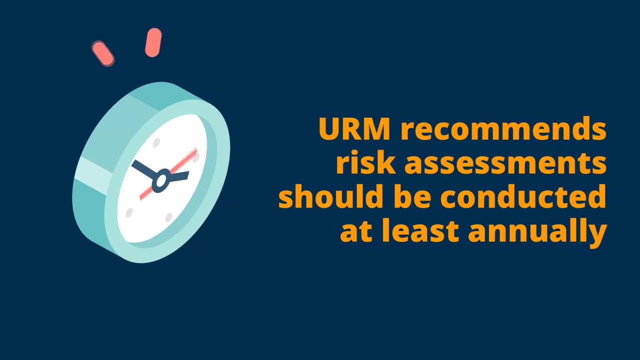 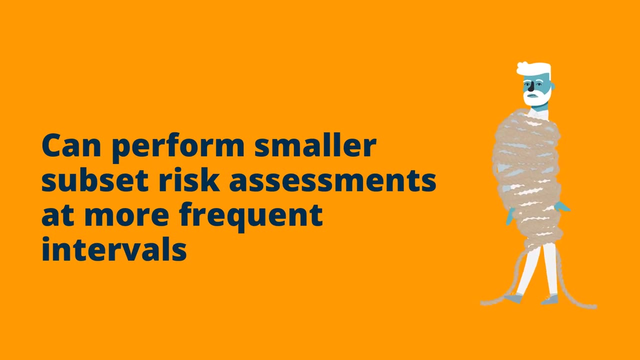 point in the year to conduct a risk assessment, although of course you can do this if you wish, it just means that each time 12 months has elapsed, you should aim to have completed the next iteration, so you could spread the workload over the 12-month period by performing smaller risk assessment on 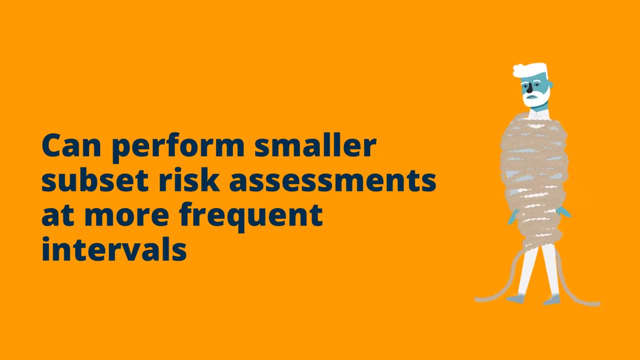 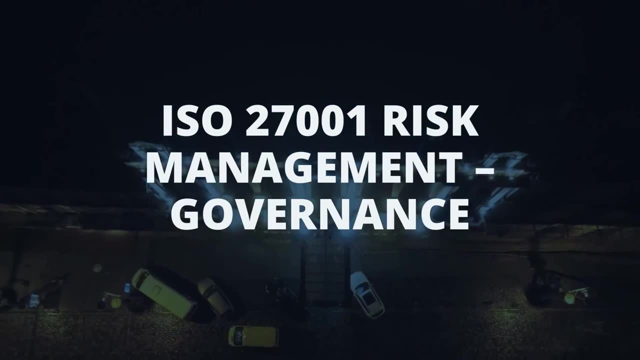 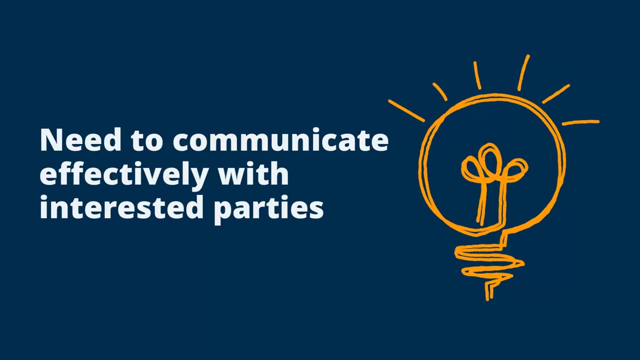 a subset of areas at more frequent intervals, if this is more manageable. ISO 2700 risk management. throughout the risk management process, you need to ensure that you communicate effectively with any interested parties. it may be useful to put together a racing raci to help you with this, as.